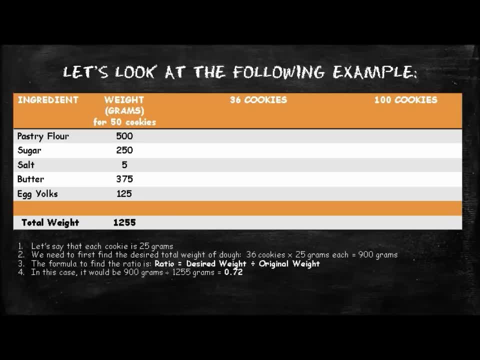 In this case, our desired weight is 900 grams. So we take 900 grams divided by the original weight of 1255 grams, and that gives us a ratio of 0.72.. You then take the ratio of 0.72 and multiply it with all the ingredients. 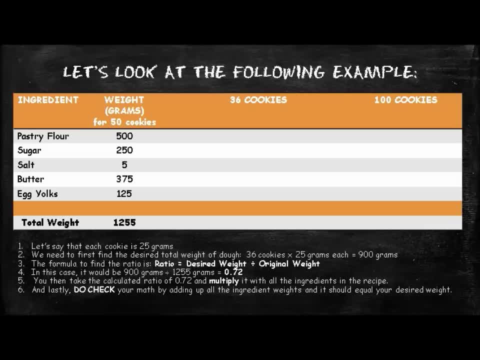 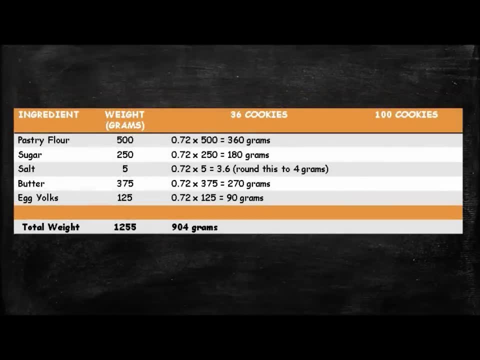 And lastly, you do need to check your math by adding up all the ingredient weights, and it should equal your desired weight With the ratio of 0.72,. let's go ahead and multiply that with all the ingredients. 0.72 times 500 is 360 grams for the pastry flour. 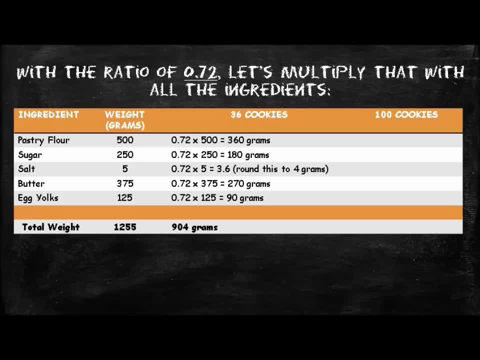 0.72 times 250 gives you 180 grams of sugar. 0.72 times 5 equals 3.6 grams for salt. Let's round that to 4 grams. 0.72 times 375 gives you 270 grams of butter. 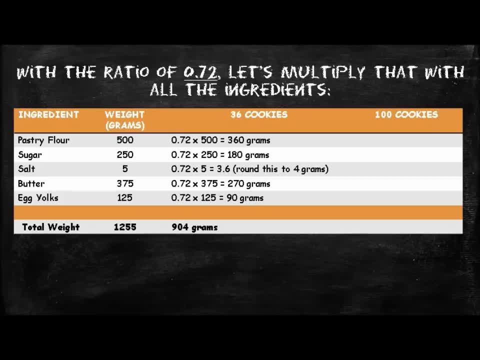 0.72 times 125 equals 90 grams of egg yolks. And lastly, don't forget to check that the ingredient weights all add up to the desired amount that you needed in the first place. In this case, they add up to 904 grams, which is very close to 900 grams that we need. 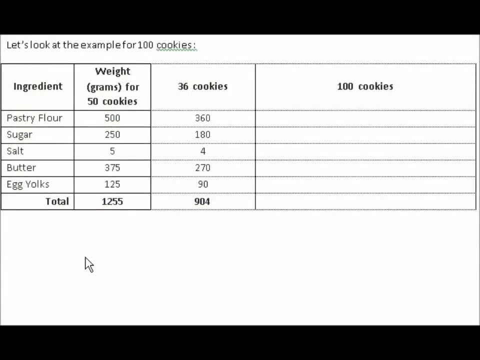 And that's due to weight. All right, now let's go ahead and try the example for 100 cookies. In this case, remember that the first thing we need to do is to figure out the desired total weights. So each cookie was 25 grams, and we need 100 cookies times 25 grams each, and that gives us a total of 2,500 grams. 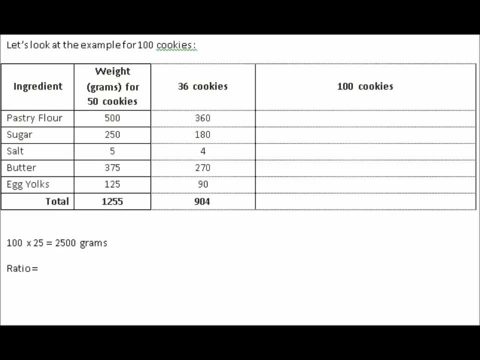 Remember that the ratio formula is the desired weight divided by the original weight. In this case, we have a ratio of desired weight of 2,500 grams divided by the original weight- right here- Of 1,255 grams. that gives us a ratio of 1.99.. 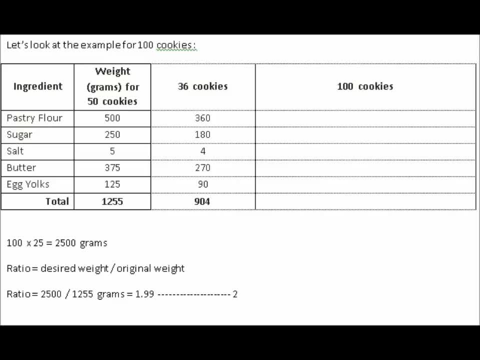 I'm going to go ahead and round this up to a ratio of 2.. It's very close to 1.99, it's a lot easier to work with. So let's go ahead now and multiply the ratio of 2 by all the numbers in the original column here.